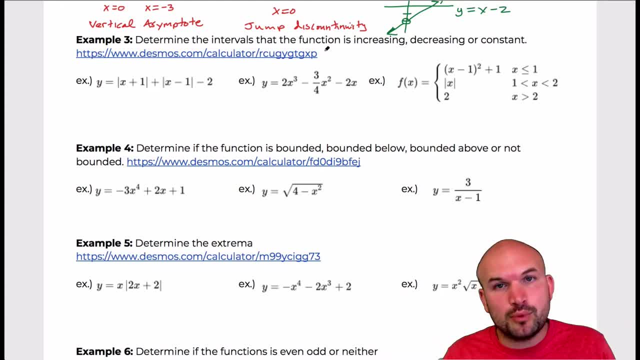 to be able to identify the intervals. Now again, it's important to understand that when we're identifying the intervals that a function is increasing, decreasing or constant, we're observing the y values to tell us if the graph is going up or down. But we are going to describe 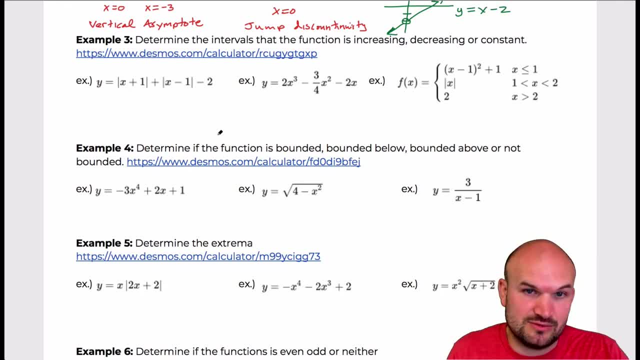 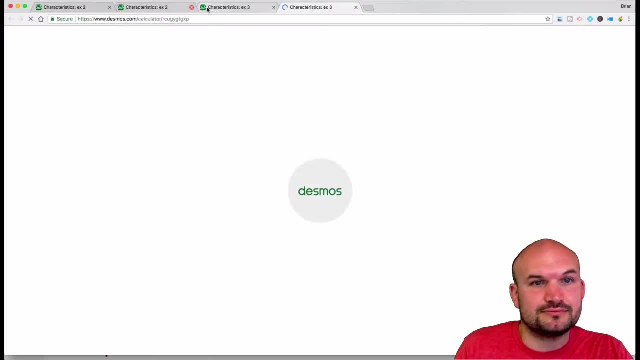 those intervals only using the x values, not the y values, And that's why I wanted to, you know, create a video like this. So, therefore, you can see the basic differences here. All right, so let's go and look at example number three, which I opened all these up for you. 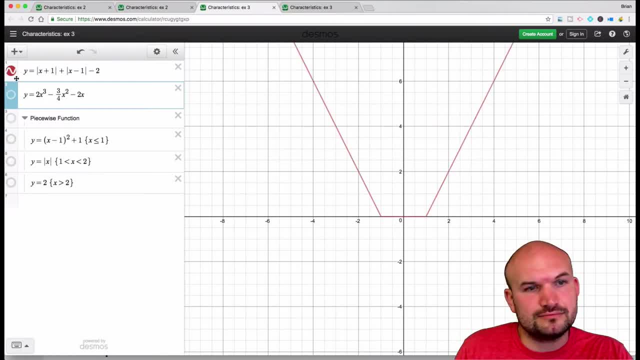 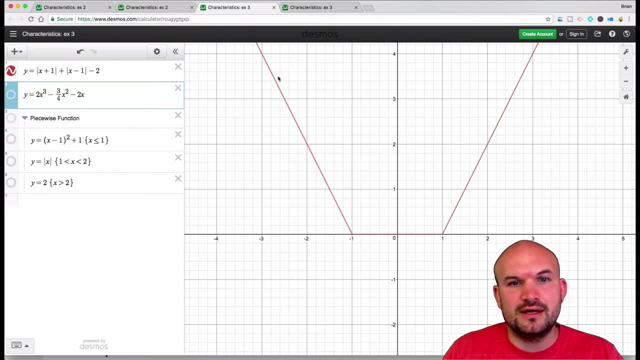 All right. so the first example: here we can see that we have this equation And it looks like. you know, as you read this graph from left to right. here the graph is: you know, as I'm looking again, you're reading it, you're reading the x values from left to right and then you're 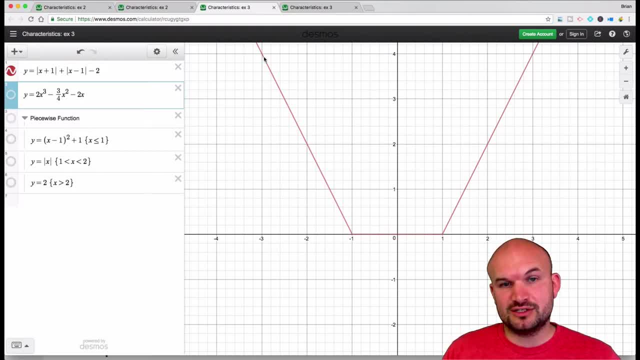 observing what is the graph doing? So from the left, it looks like the graph is going down all the way down to negative one. Then, from the interval, from the x interval of negative one to one, the graph is remaining the same. And then, from the left, it looks like the graph is going. 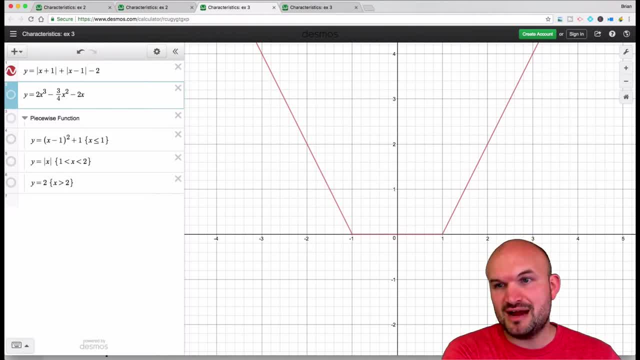 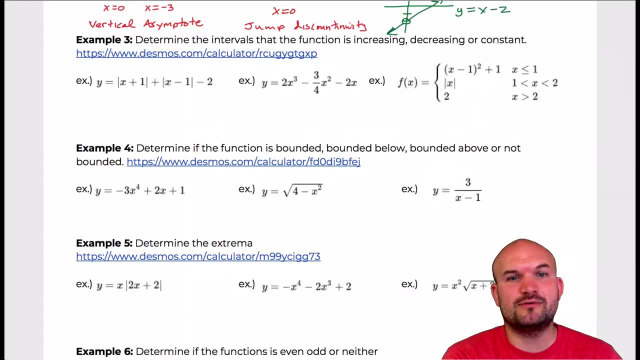 down from the interval, from one all the way to infinity right, Because this graph doesn't look like it's stopping. the graph is going to continue increasing. Okay, So the way that we would just kind of write that is: let's go and use purple So we can say that the graph is, let's go and do. 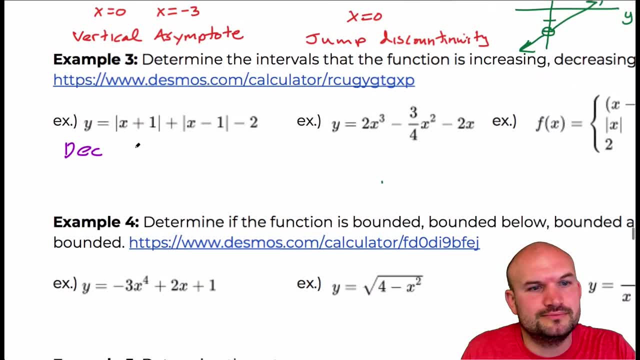 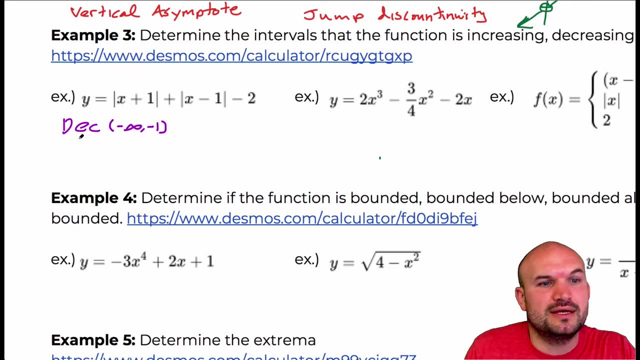 decreasing first. So the graph is decreasing on the interval of negative infinity to negative one. It's constant On the interval from negative one to one. And again I'm using open parentheses because you know, technically at that point it can't be at the point like negative one. 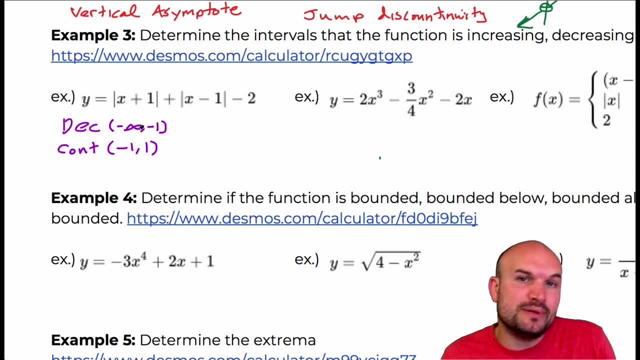 it can't be decreasing and constant at the exact same point. So we're using the open and interval. So therefore we're not like cross cross defining the values And then we can say that the graph is increasing on the interval one to infinity. Alright, so let's go and look at the 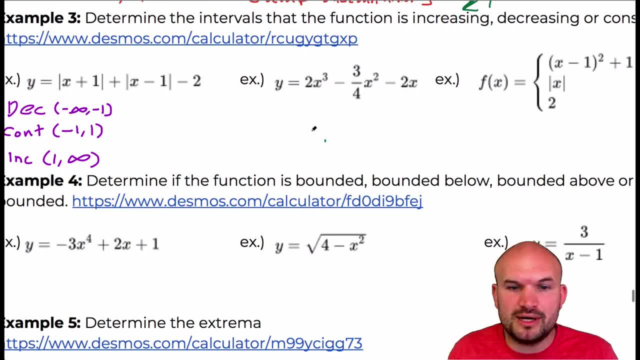 next one here, which is a. let's go and look at the next one here, which is a let's go and look at the polynomial, which we'll talk about again. So, looking at the polynomial, see, okay, pulls back. 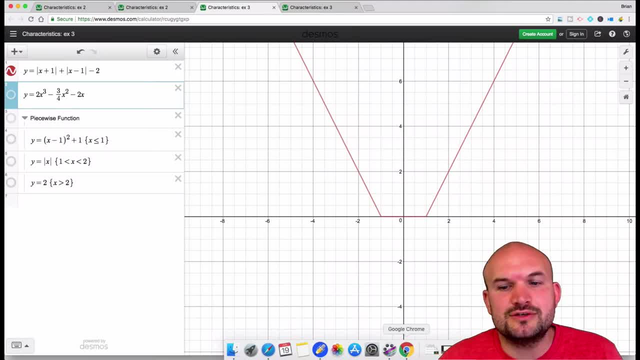 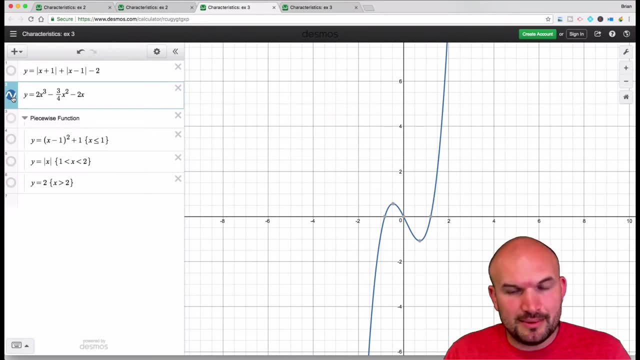 up. So now we can look at this. And let's look at this next equation: polynomial boom. Okay now I like this equation because obviously this is one that you can easily graph like in a graphing calculator, And I prefer Desmos working on this one, just because it's so easy to find these. 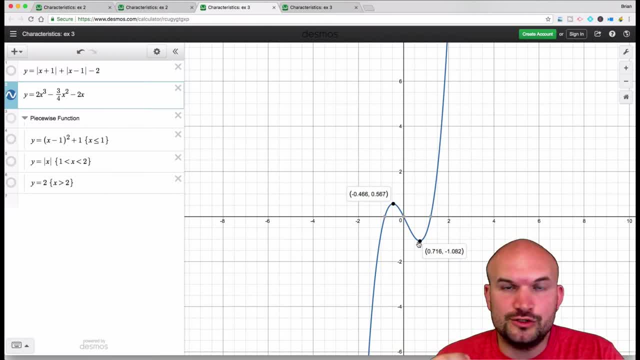 absolute maximums and absolute minimums having to use graphing technology. But you could use graphing technology- you know TI, calculator or Casio or whatever you use to find those values. But once you find those values, it's very important. 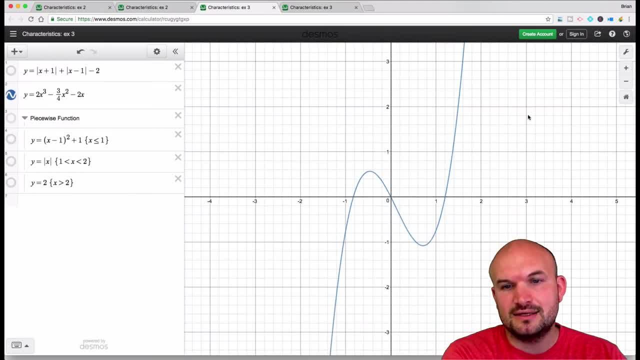 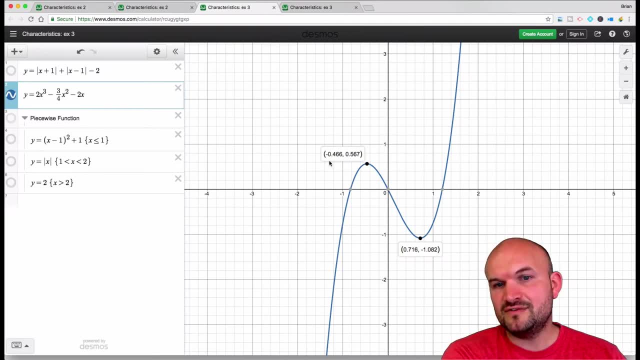 to remember that we are looking to extract only the x values, right, So we can see from negative infinity to negative 0.466,. the graph is increasing. the y value is just telling us, like, how high that point is going. but that's not going to be how we're going to describe it, So we're going to 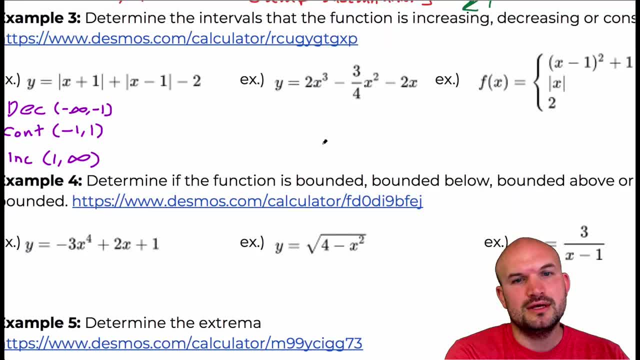 describe the increasing decreasing intervals. So in that graph it was increasing to decreasing and then increasing back again. So let's go ahead and write the intervals increasing first. So it was increasing Now. I wrote these down because I was like I'm not going to remember these, So it's. 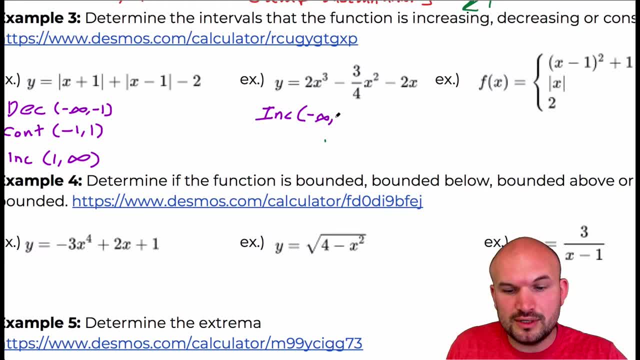 increasing from negative infinity to negative 0.466.. Then I'm going to use a union symbol. And then it was also increasing on the interval negative- No, I'm sorry, not negative- 0.716 to infinity. That looks really bad. Sorry about that. And it was only in decreasing, If you remember. 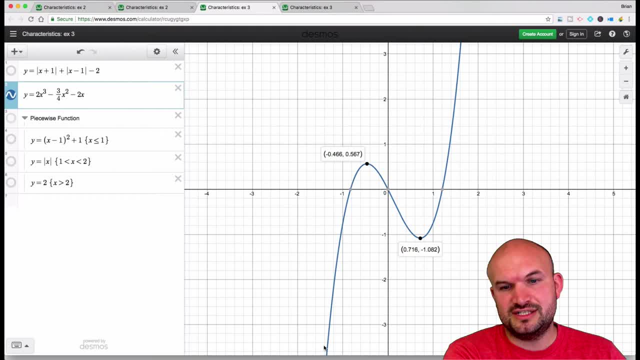 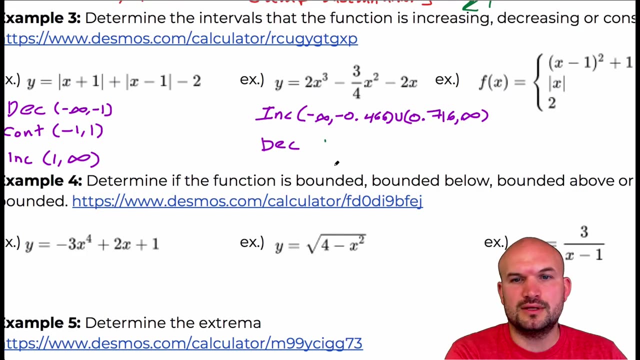 let's look back at it again, Right? So it's increasing from negative infinity to negative 4.66.. And then it's increasing from 0.716 to infinity, And then it's decreasing from negative 0.466 to 0.716.. So therefore, we can say that it's decreasing on the interval negative 0.466 to. 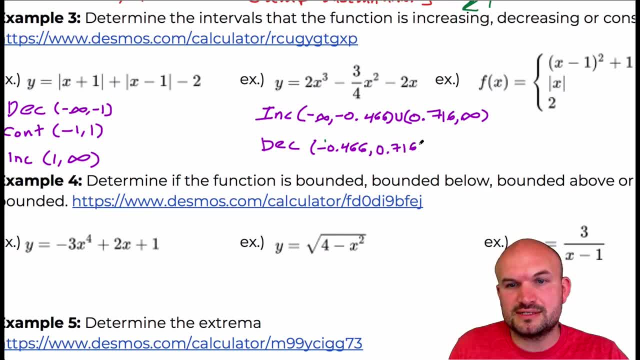 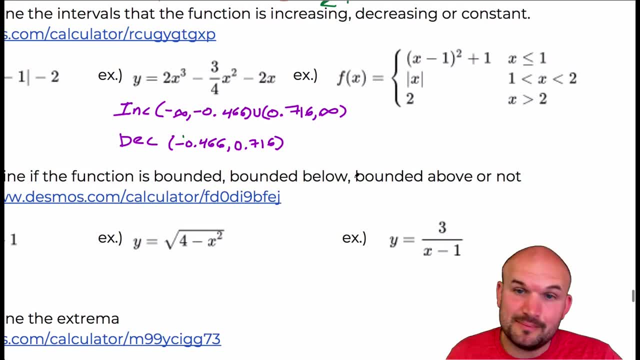 the interval 0.716.. Okay, Again, you don't need to use the union symbol, but I think that it sometimes kind of helps. All right, The last example is a piecewise function. You can see again that we have a function that is defined for three different functions. So we're going to. 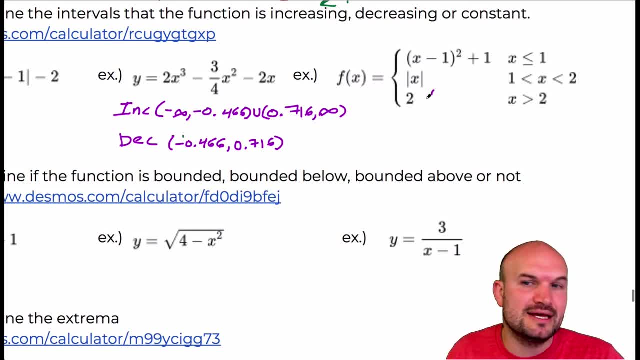 we have a quadratic, an absolute value and then a constant And basically what we you could probably go ahead and define. if you understand, know what these graphs look like, You could probably define the increasing, decreasing values just by looking at this piecewise function. 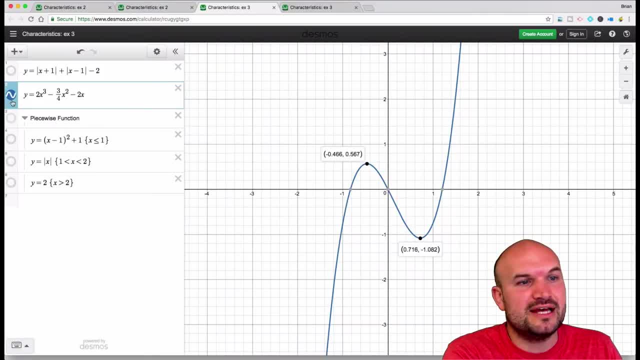 But I know that's not something that many people might be as comfortable with. So I wrote them all out as piecewise functions So we can look at them all together. All right Now. in this case you can see, here we have the quadratic and then we have the linear equation. 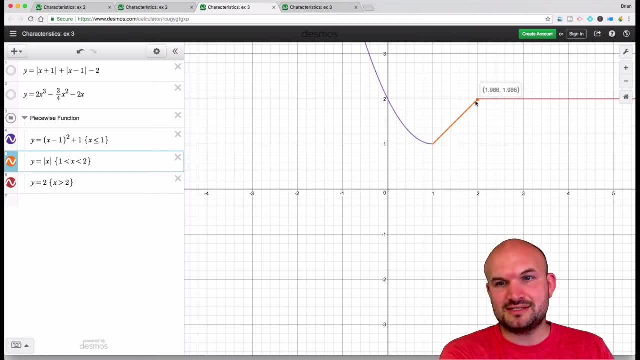 And then for then we have the constant. Now it's important to kind of note that the Desmos is not really giving us an accurate answer. It's giving like 1.22, or it's getting close. Here I'm trying to get really close and it's kind of hard, But you can see, at one it's. 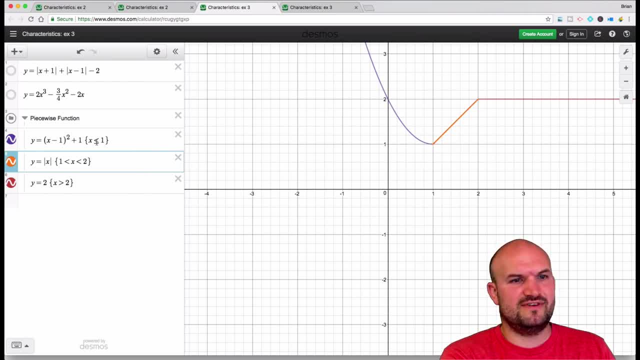 should be undefined At one. it's defined for that. I'm not sure why that's giving me that, because it should be defined for there. Oh, I guess it depends on the function. But sometimes you can get a little bit difficult. You can get like really close to there and it won't be able. 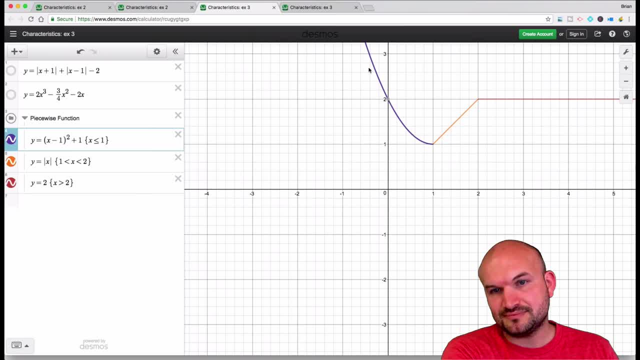 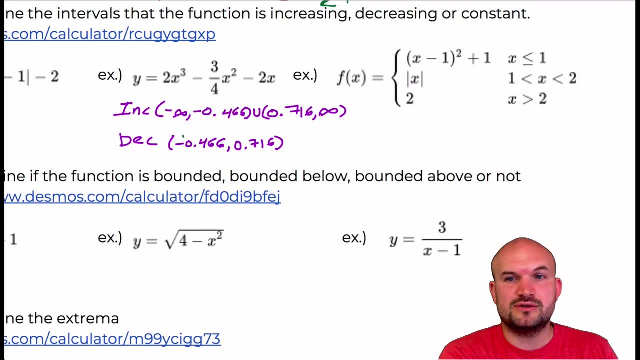 so just be aware of that. But we can see that the graph is decreasing from negative infinity to 1.. It's increasing from 1 to 2, and then it's constant from 2 to infinity. So we're just going to go ahead and write that down. I think I can remember all that, hopefully. 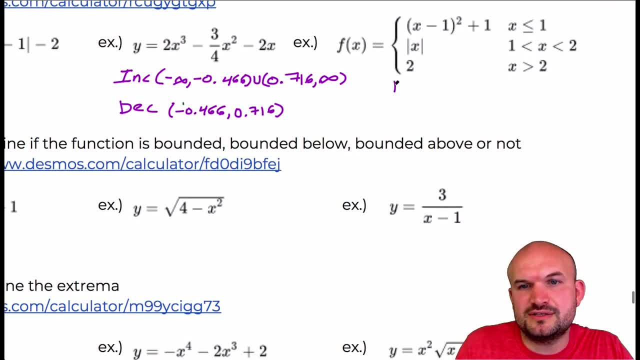 Let's go and check it out. So let's say it was decreasing first. So we'll write decreasing from negative infinity to positive 1.. It was increasing from positive 1 to 2, and then it was constant from 2 to infinity. And again, this is a good description. 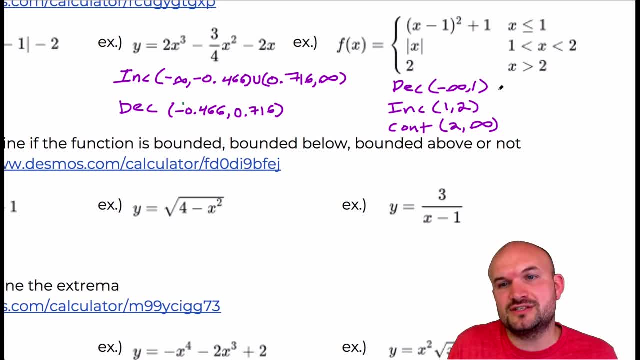 of the x values At each of those intervals, we can say that the graph is going. you know, I didn't do this before. graph is going down On the interval 1 to 2, the graph is going up On the interval 2 to infinity. the graph is constant. So when we're describing these intervals, 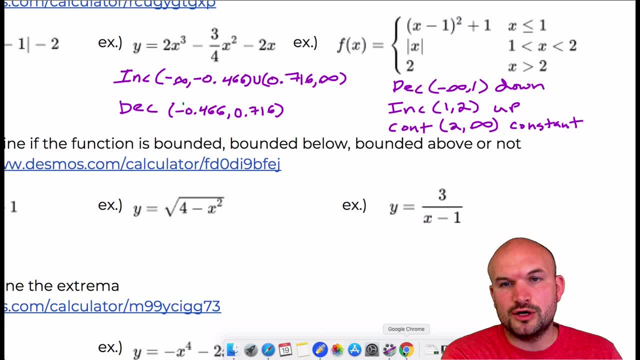 again. I just want to write this in there: When we're describing these intervals, you know we're not describing how high or how low, or you know what value is staying the same. We're just describing it's going down on this interval. 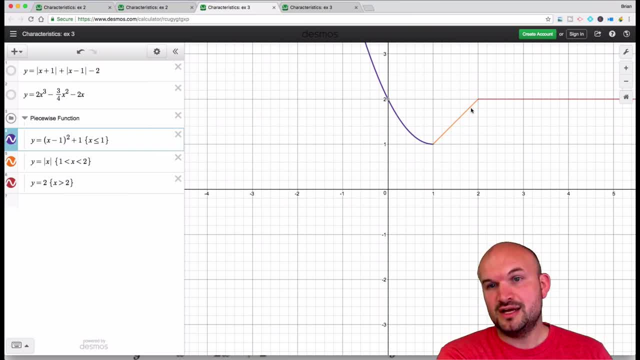 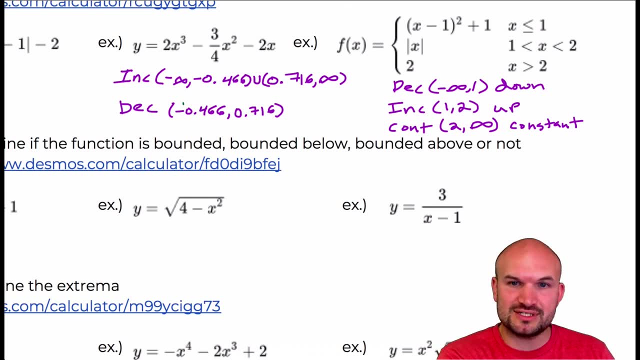 from negative infinity to 1.. It's going up from 1 to 2, and it's remaining the same from 2 to infinity. So there you go, ladies and gentlemen. That is how you describe the constant intervals when given an equation. Thanks,